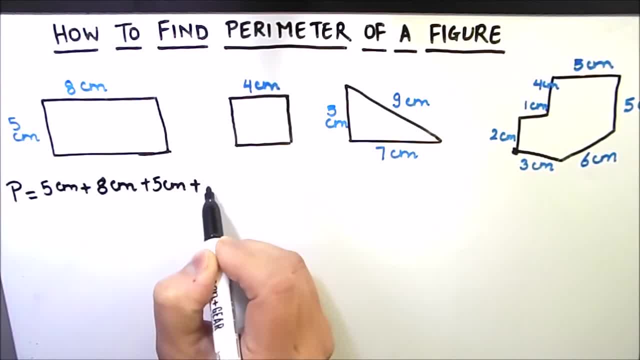 because opposite sides are equal in rectangle And the base is 8 centimeter length, We will add all the four sides, So this is going to be 8 plus 5 is 13, and 8 plus 5 is 13, and 13 plus 13 is 26 centimeters. So the perimeter of this 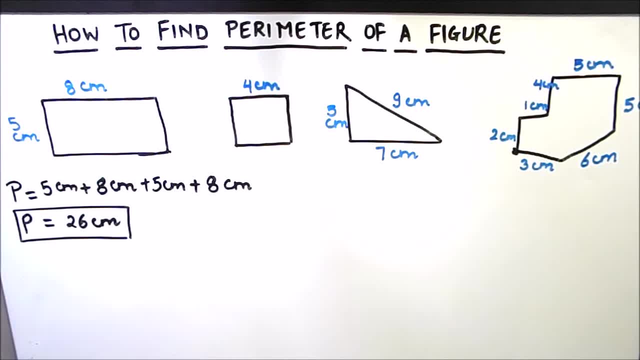 rectangular field is 26 centimeter. Perimeter is same as the unit of length we are using, So here it is centimeter. Here we have taken two times length and two times breadth, So the formula for perimeter of rectangular field is two times. 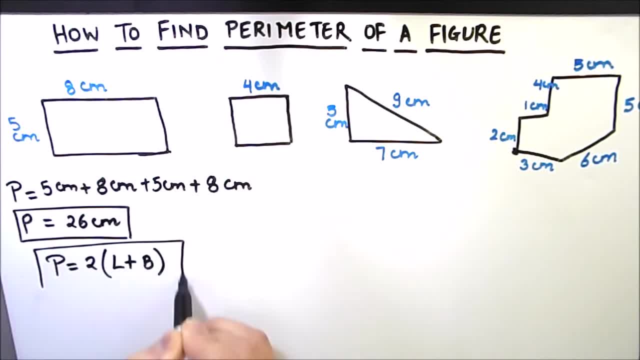 length plus breadth. This is the formula for finding the perimeter of a rectangular field. Let us now find the perimeter of the next picture, which is a square. So square is a figure having all sides equal. So we need to add 4 centimeter four times to get the perimeter of this figure. 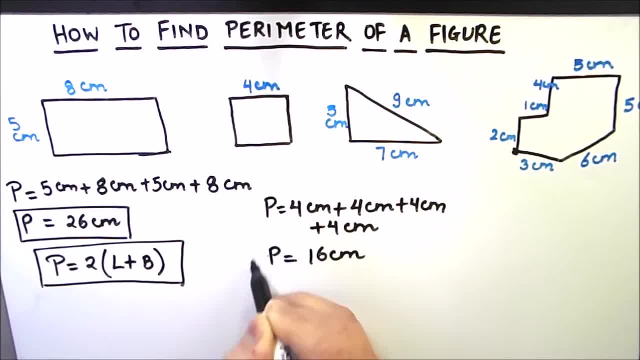 The perimeter of this square is 16 centimeters. The formula for finding the perimeter of square is 4s, where s is the length of side of the square. Next we have triangle. For the perimeter of this triangle we will add all the three sides. So first is 7 centimeter, then 5 centimeters and then 9 centimeters. 7 plus 5 is 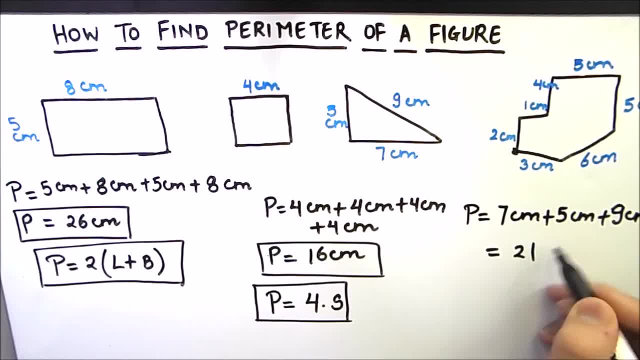 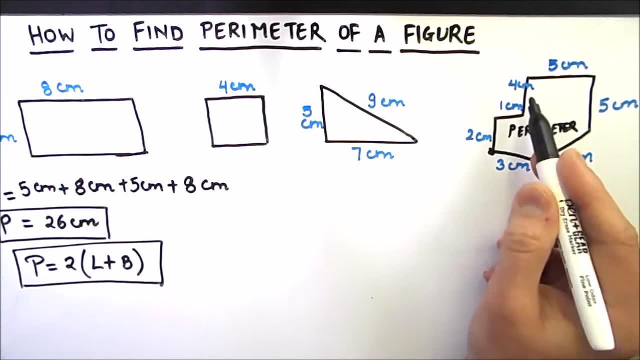 12, and 12 plus 9 is 21 centimeters, so the perimeter of this triangle is 21 centimeters. for finding the perimeter of complex shapes, we should start with one side and should go around the figure, adding the sides one by one. so let us start from here. so this is: this side is 2 centimeter. 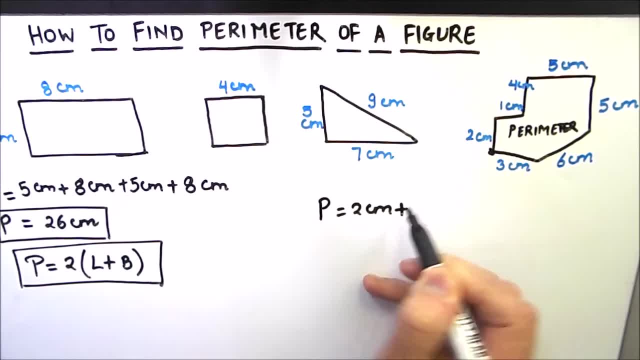 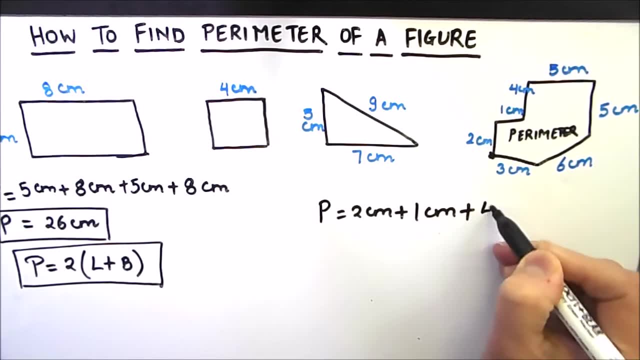 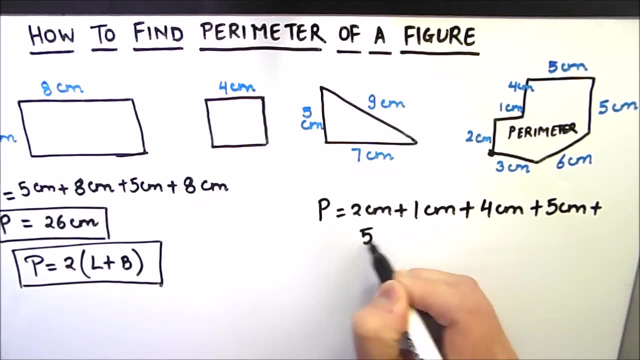 so 2 centimeters plus. then this is 1 centimeter plus 1 centimeter, then 4 centimeters. up top is 5 centimeters. again this is 5 centimeters, then 6 centimeters and then 3 centimeter. we come back to the same point. so this is how you should.